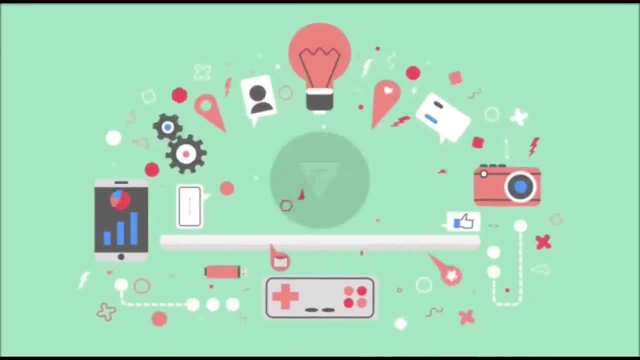 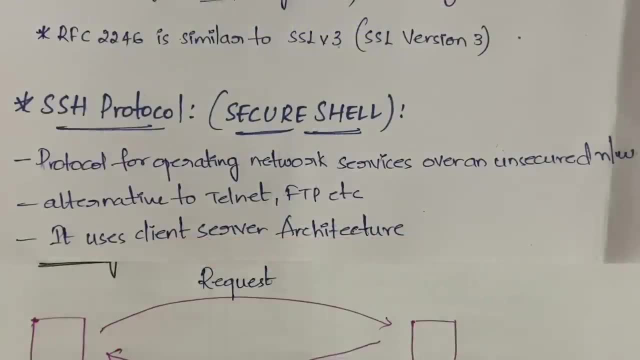 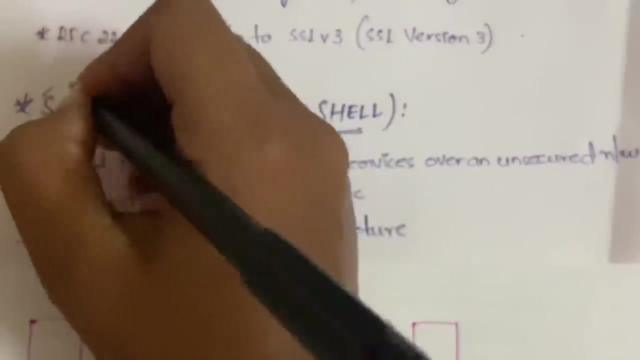 Hello everyone, welcome back to my youtube channel, travel free. In this video, I am going to explain you about the SSH protocol in the subject of network security. First of all, SSH means secure shell protocol, S is for secure, SH is for shell, secure shell protocol Got. 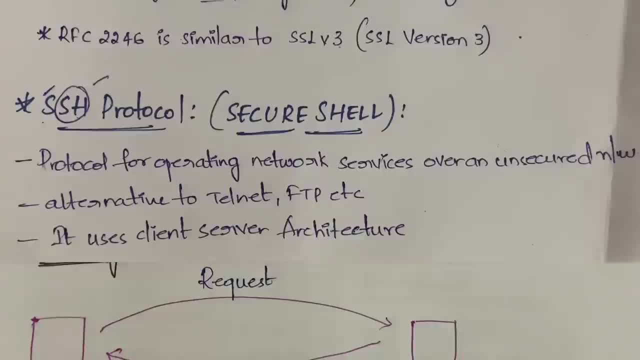 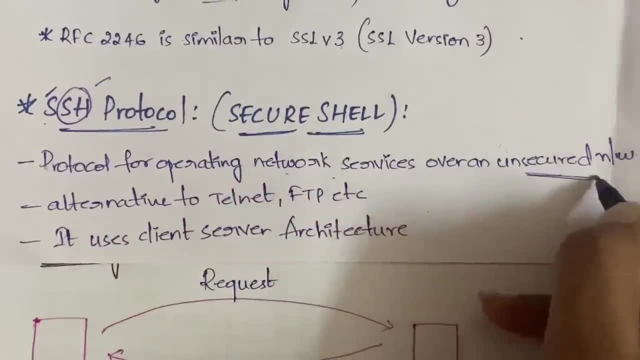 it. So here, why do we use this protocol? and what is the working of this protocol? everything I tell you. So, basically, it is a protocol for operating network services over an unsecured network. So if you are having any unsecured networks, then in that case we will have some. 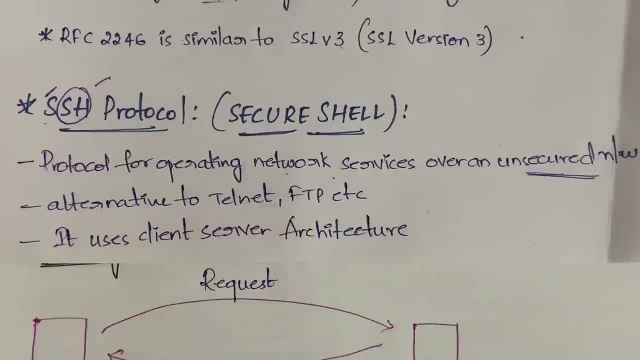 you know we cannot easily enter that network because we know that it is unsecured network and our data may be lost in that. So in those kind of unsecured networks also we can go and we can access. we can access the services of those kind of unsecured networks with the 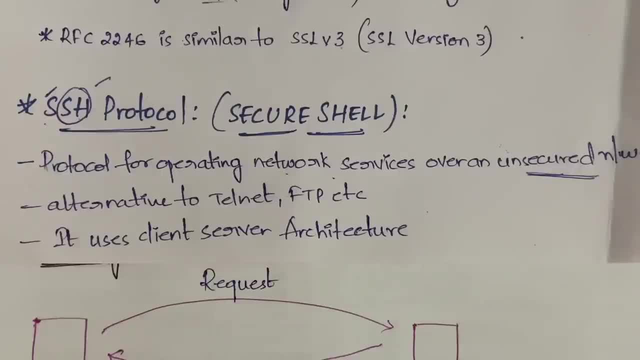 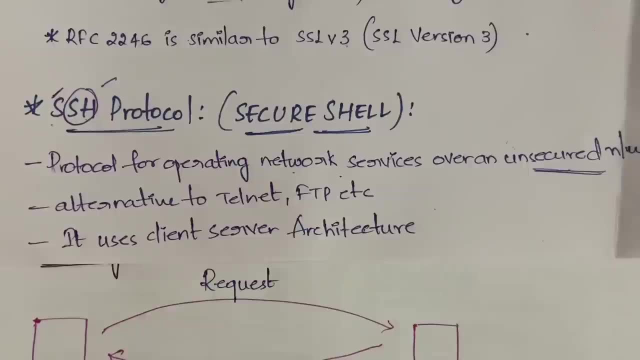 help of this secure shell protocol Got it. So it is an alternative to telenet and ftp. Not only telenet ftp, there are so many other protocols also, So it is an alternative to telenet ftp, smtp, so some other protocols also, Because they are not more secured, you can. 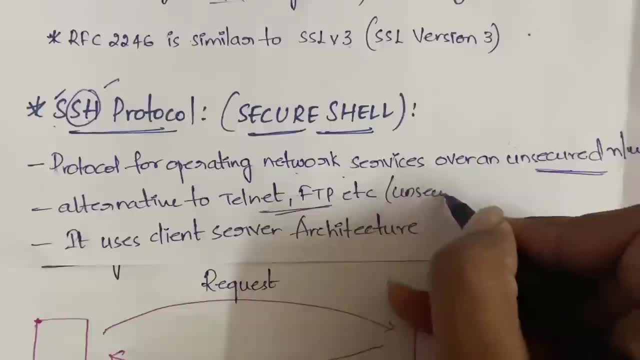 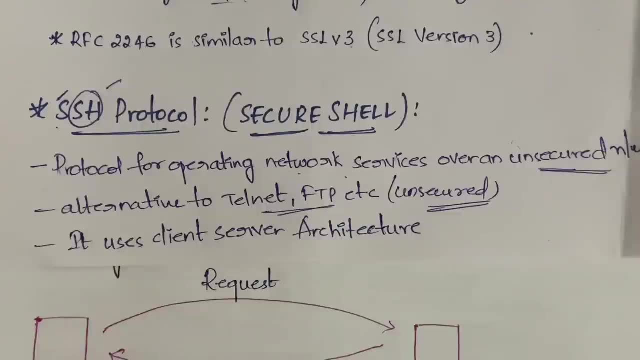 say telenet, ftp, are unsecured protocols when compared to secure shell. Secure shell protocol Got it. And here we use the concept of client server, We use the client server architecture, Got it. So secure shell protocol is nothing, but it is basically. 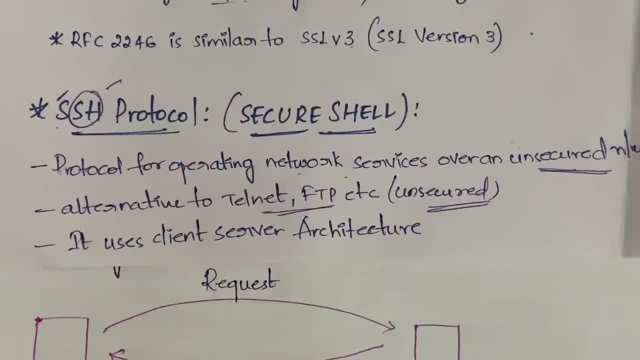 a protocol through which you can access the services of an unsecured network securely, that is, without any fear, without any hesitation, without any worries that our data may be lost or our data may be, you know, stolen, or our data may be modified. We can happily use the. 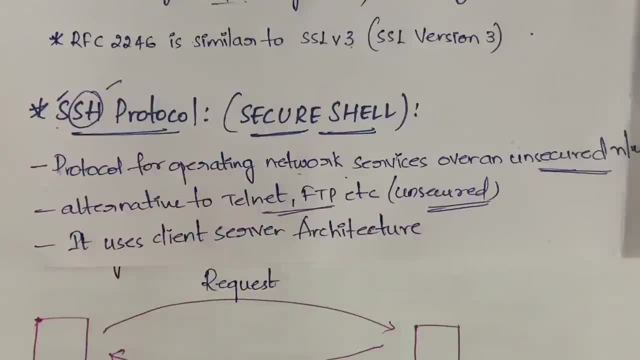 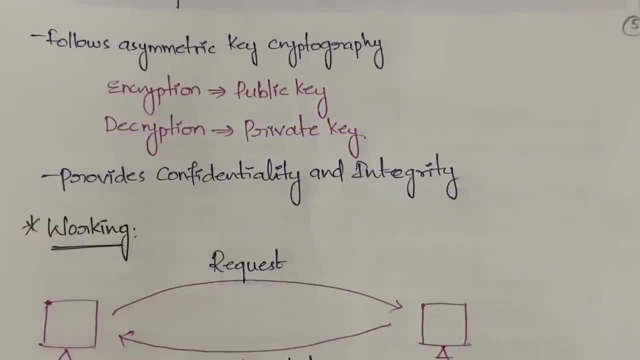 services of an unsecured network. We can access the services of an unsecured network without unsecured network. also with this SSH secure shell protocol Got it And it follows the client server architecture. And also one more thing is that it follows asymmetric key cryptography. You 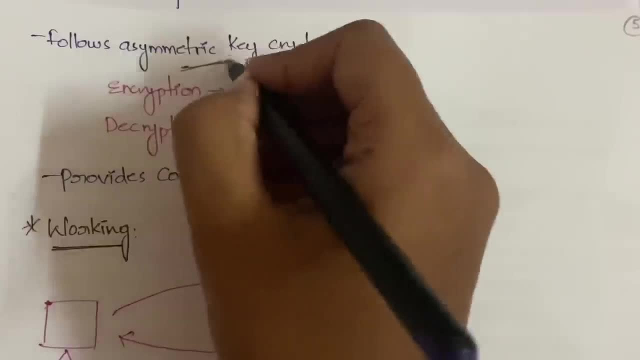 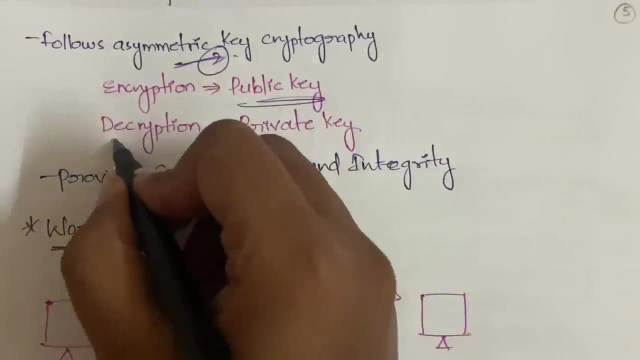 know what is asymmetric key cryptography? right, You will be using two types of keys: at encryption, one key and for decryption, one key. So at encryption end, we are using the public key and on the decryption end, we are using the private key. Got it? So this is about the 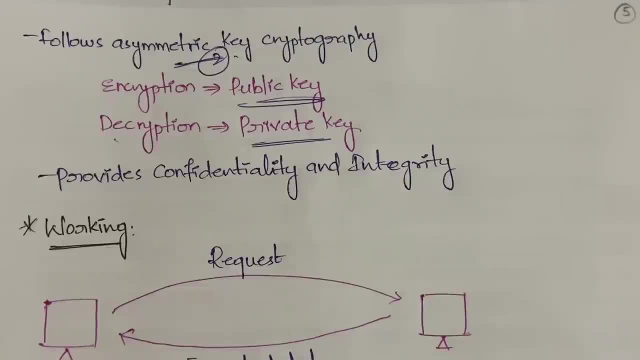 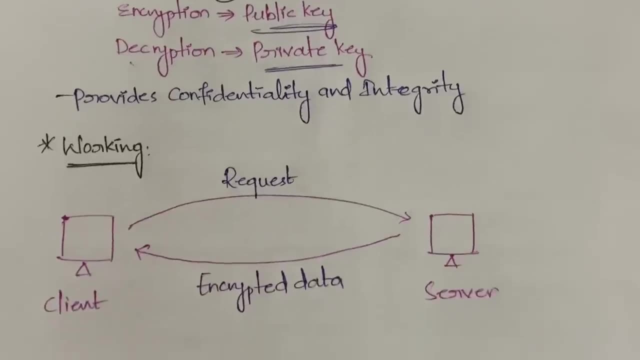 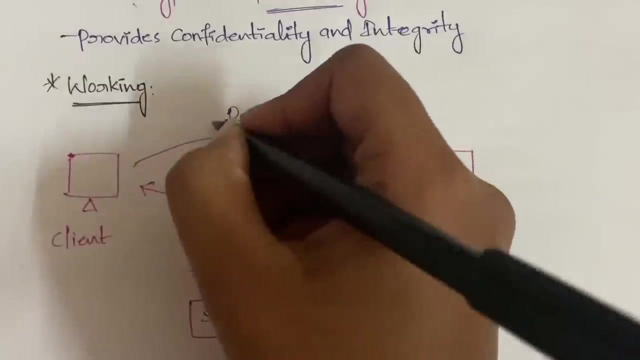 keys used by this secure shell protocol, and this is for providing confidentiality and integrity of the data. Got it. Now let us see the working, which is very important. So, first of all, what happens is the client will request the data to the server, That is, the client will send the request to the. 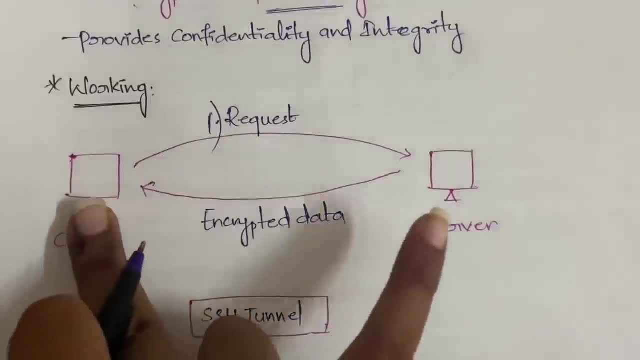 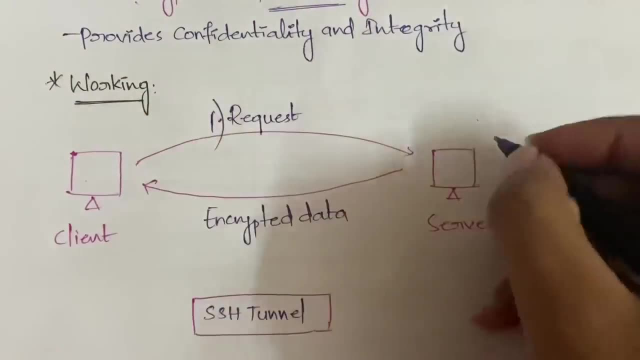 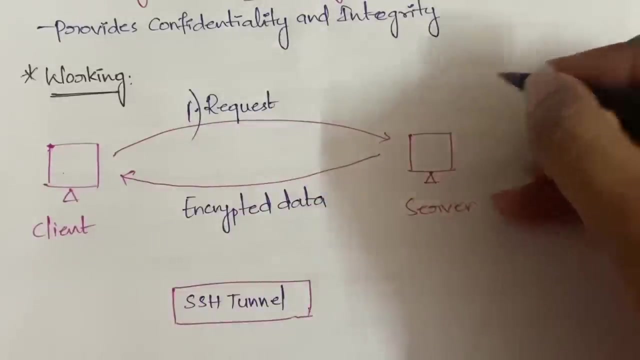 server. This is the first step. The request is sent from the client's end to the server end. Now what server will do? Once request is sent, client's work is done. Now the complete work server has to do. What server will do is it will check the authentication of the client. 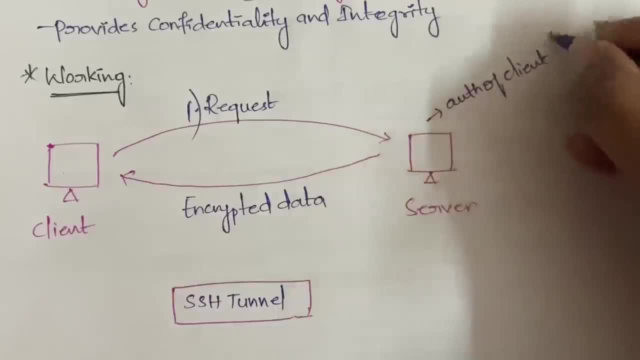 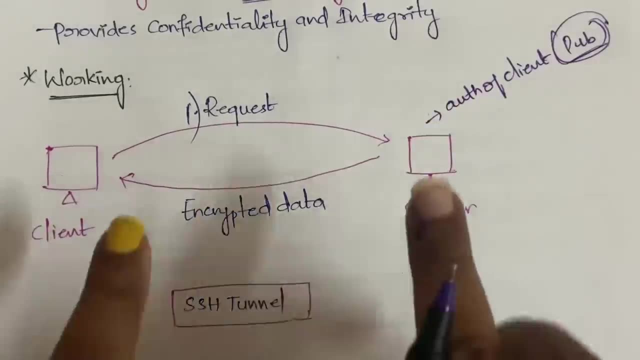 Authentication of client is checked first. How? With the public key? It will check the public key of the client because the public key is same for everybody, Right? The public key is available to everybody, Right? So it will check the public key of the client, whether the public key is correct or 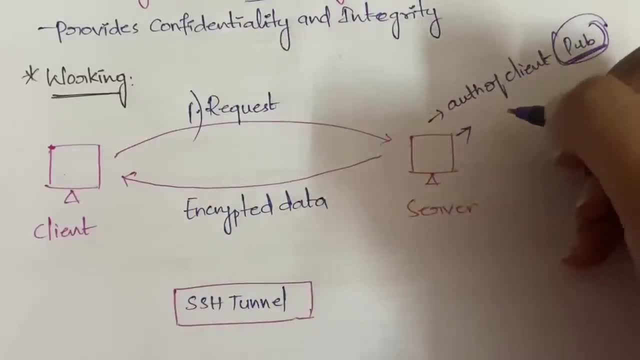 not Right? Okay, Public key is checked. Second, what it will do: once it identifies that the public key is matching the public key is correct, then it will generate a random string, Any random string message it will generate. Okay, And this random string is sent to. 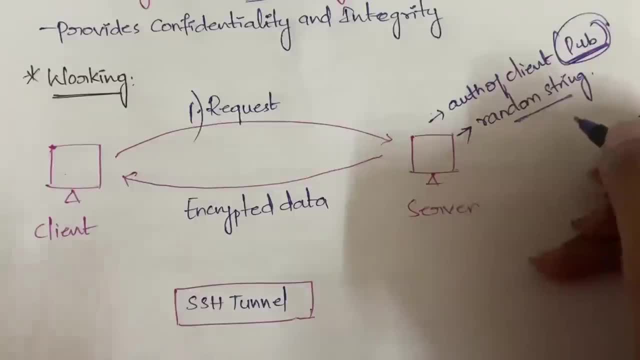 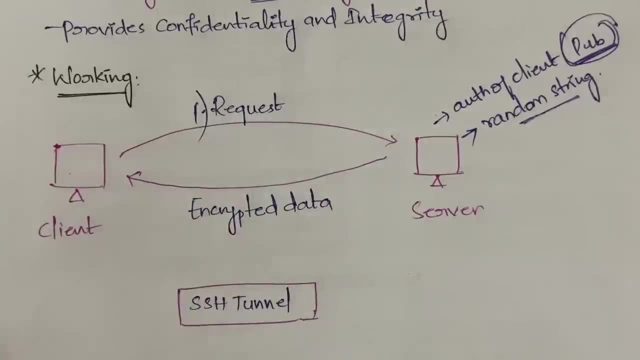 the client. This random string is not the data which the client has received, So the data is not actually transferred here. Right, This is only for the checking, the authentication between the client and server. That's all Got it. Now a random string is generated from the server's end and this random 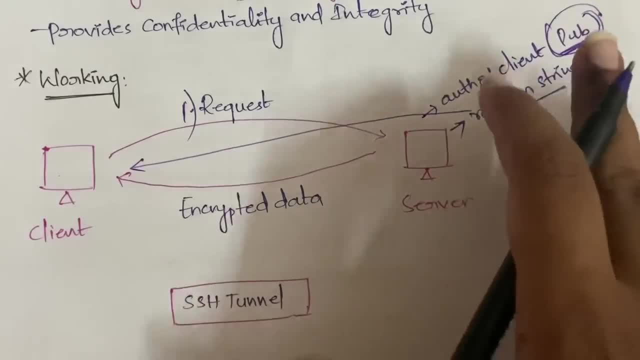 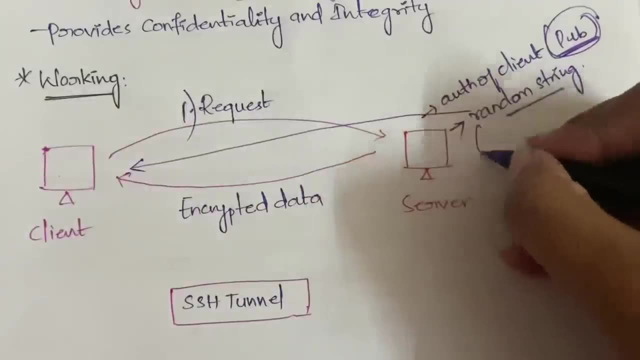 string is sent to the client. Got it? So the random string which is generated by the server is sent to the client. Now what happens? Yeah, Sorry, Sorry, Sorry. Before sending the random string, it will encrypt this random string, Just like a normal text. it will not send, It will encrypt it and it will. 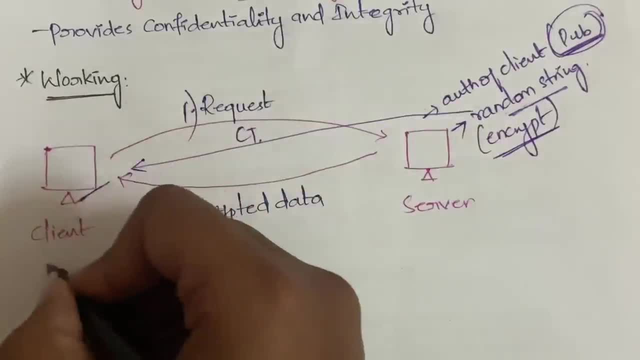 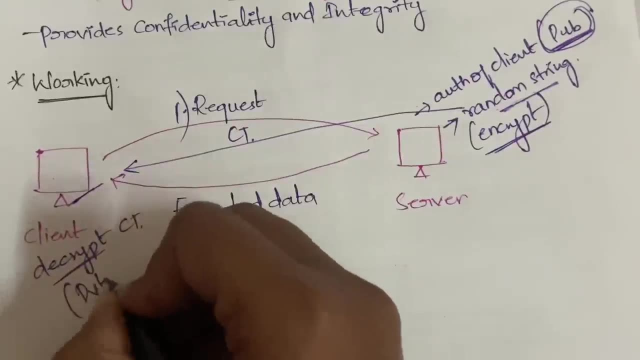 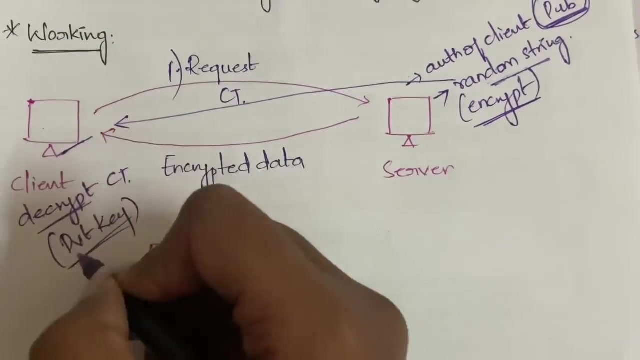 send the ciphertext to the client. Now, what client will do? The client will decrypt the ciphertext which is sent by the server by using the private key of the client. So decryption we are doing with, as I already said, decryption. So here the client will decrypt the data with the help of its private 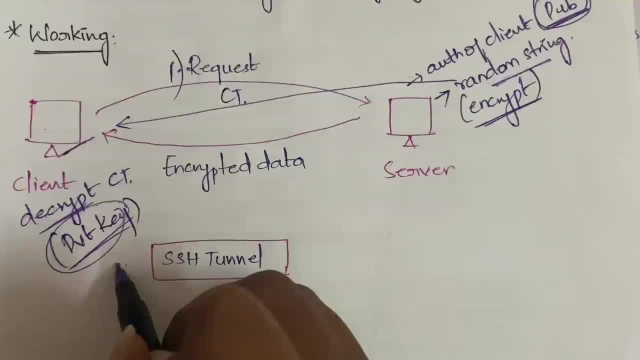 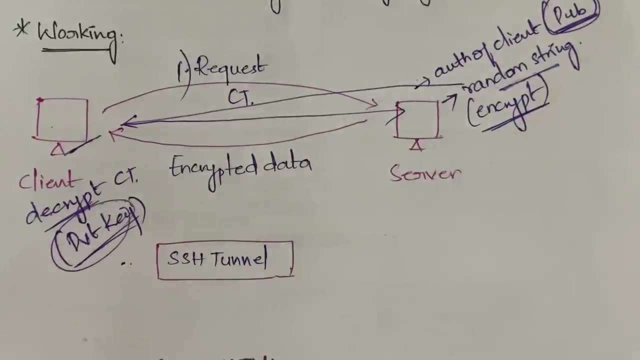 key, Got it. Now the client will decrypt the data and again send back the decrypted data to the server. You know this decrypted data will act as an acknowledgement, So once the decrypted data is sent back to the server, the server will get to know. Okay, So this is what I have sent and the 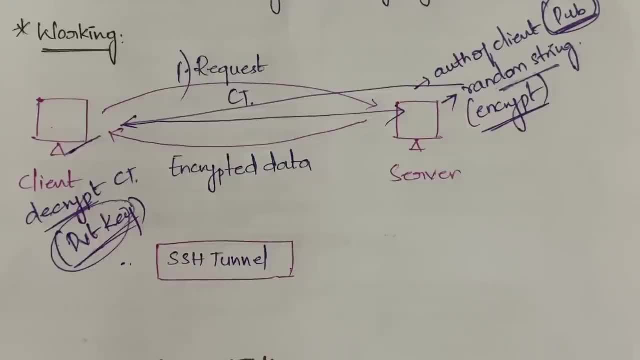 client is able to decrypt it correctly, That is okay. He is a, or she is a, trusted client, Right? So the keys are matching, everything is correct. So that is why he is able to decrypt it perfectly, Okay, Fine, So now I can trust, Right? So now what happens is: 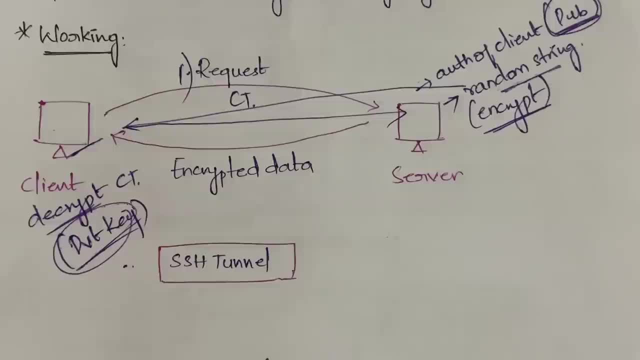 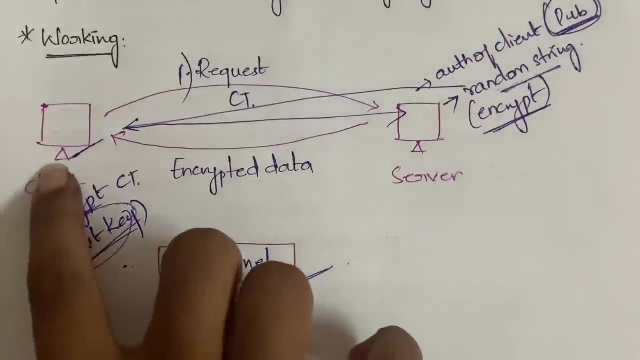 finally, once the authentication of client is proved, the authentication of client is confirmed on the server's end. Now SSH tunnel is created. Okay, So what is this SSH tunnel? It is a channel for communication between the client and server. So now, whatever data client wants, or whatever data, 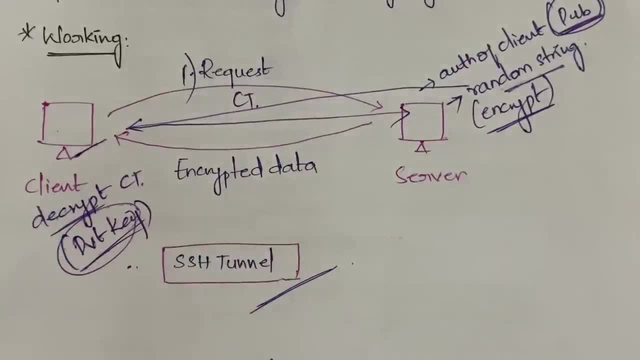 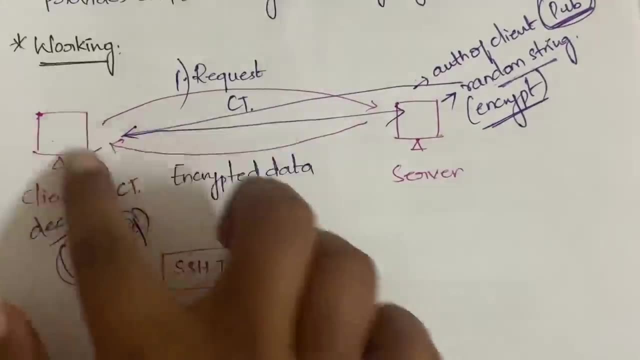 server wants to give will happen through this SSH tunnel, That is, it is very secure. Nobody can enter into that tunnel and steal the data. Okay, So in order to establish this tunnel, this is the process we need to follow. First, client will send the request Now in order to check the authorization. 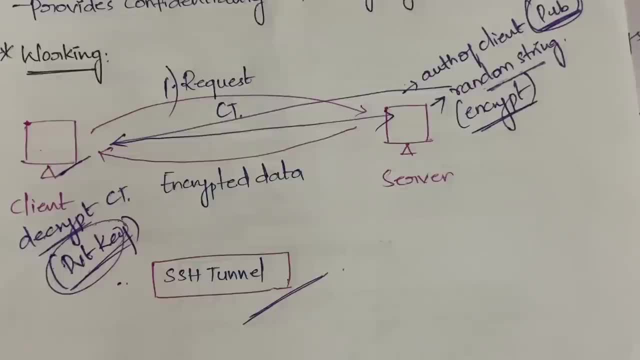 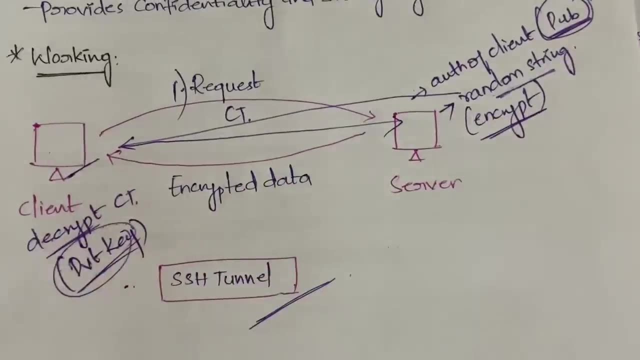 of the client. it will check the public key, If the public key is matching, and it will generate a random string and it will encrypt that random string with the help of the public key which is on the server's end, and that will be sent back to the client. Now what client will do? Client will 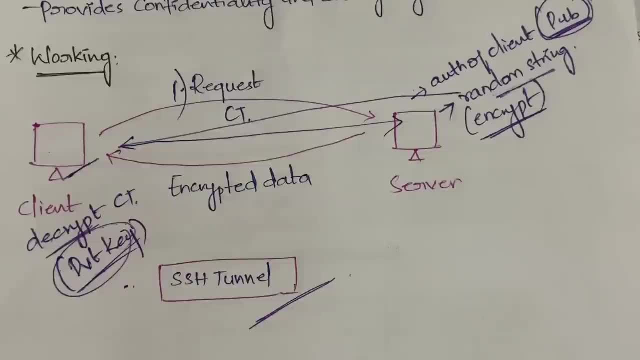 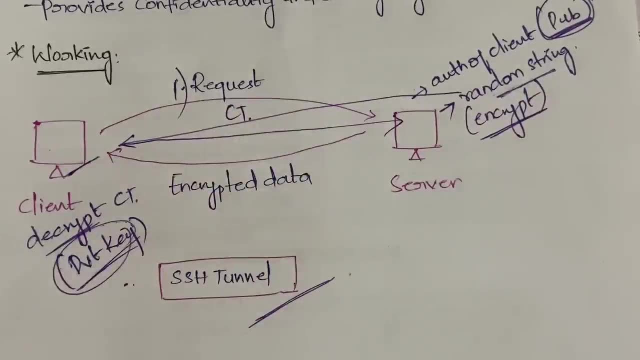 decrypt the data with its private key. Now, once decryption is done, it will send back the data to the server. If the data is matching, then the server will confirm the authorization of the client and then a tunnel is created. In that tunnel, the communication between the client and server will. 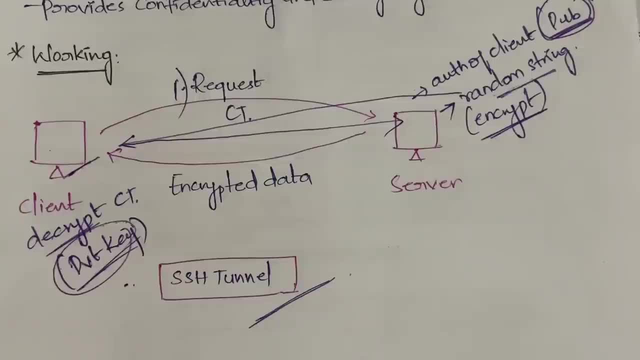 take place. Okay, So this is all about the secure shell protocol. I hope you guys are clear with what I have explained in this video. If yes, hit the like button and also share it with your friends. and if you are having any doubts, 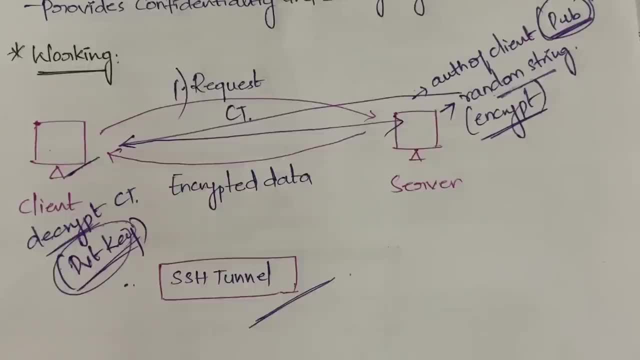 you can ask me in the comment section or I will give you my contact details in the description. You can contact me through my Instagram or Gmail. Okay, So let's meet up in the next coming video with another topic. Thanks for watching the video till the end.